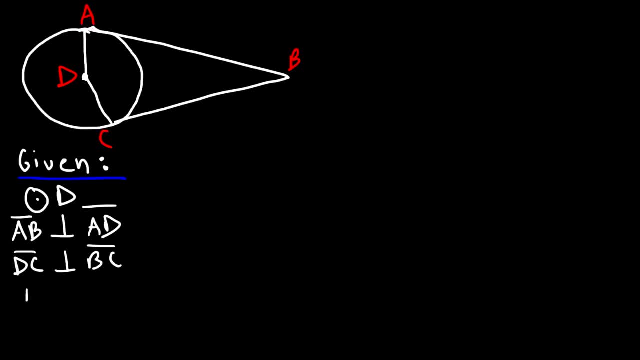 So, with this information, prove that AB is congruent to BC. Feel free to pause the video and try this problem. So let's make a two column proof: S for statements, R for reasons. So the first statement we could say is that D is the center of the circle. 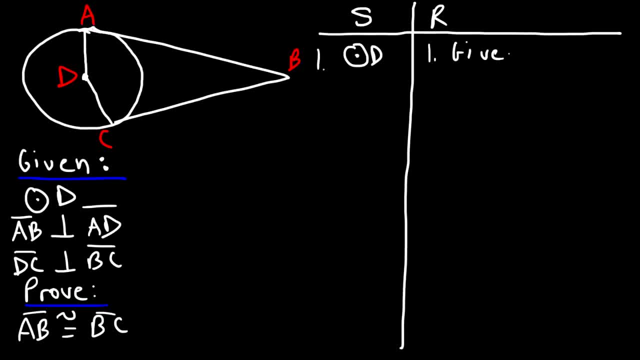 And so this information is given to us Now. in step two, we could say that AD and DC are congruent. Now let's look at step three. Now, since D is the center of the circle, that means that AD represents the radius of the circle and DC represents the radius of the circle. 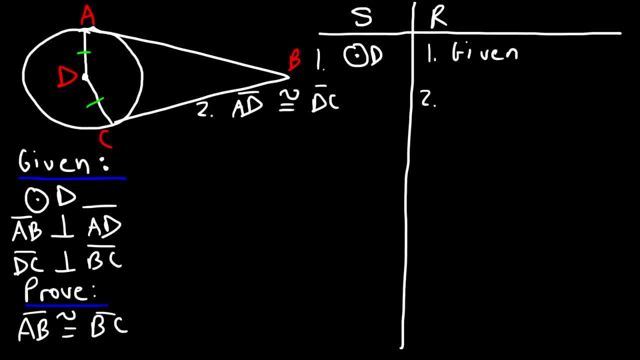 Because the radius is the distance between the center of the circle and any point on the circle, And so the reason for this. we could say that all radii of a circle are congruent. Now, what else can we say? The next thing we could talk about is the other given statement. 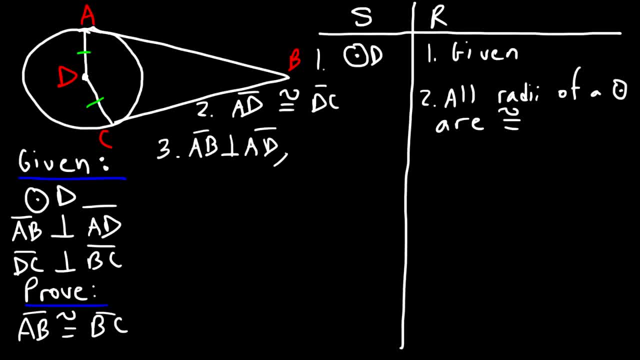 That AB is perpendicular to AD and also that DC is perpendicular to BC, And so we could just write given for that step. Now, any time you have two perpendicular segments, you need to know that they form right angles. So in step four we could say that angle A and angle C are congruent. 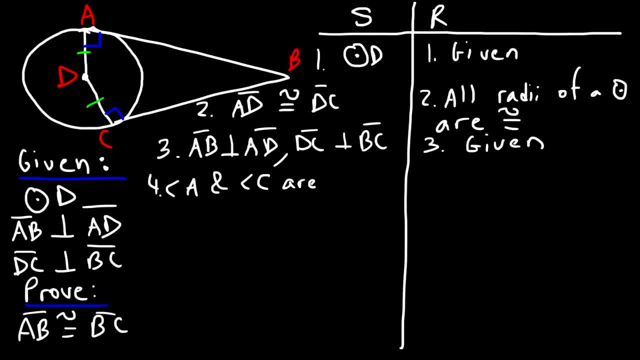 And angle C are right angles, And so we could say this is a definition of perpendicular lines. Perpendicular lines form right angles. Now step five. we could say that angle A is congruent to angle C. And the reason: right angles are congruent. 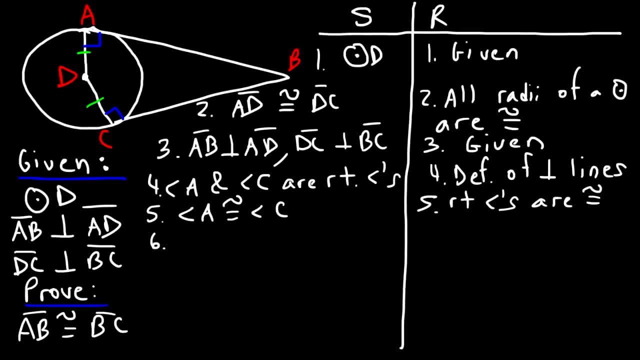 To each other. So now step six. We could say that BD is congruent to itself, And this is due to the reflexive property. And so now we have enough information to prove that the two triangles are congruent And we can use the hypotenuse leg theorem.